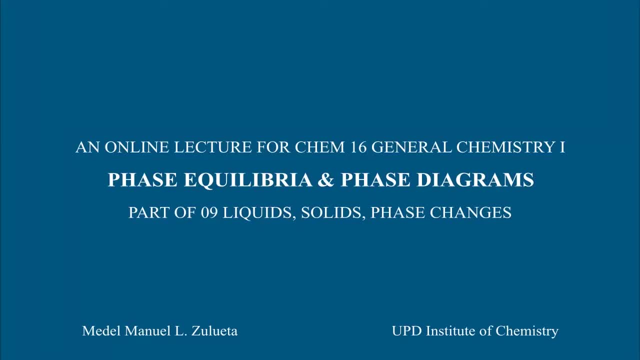 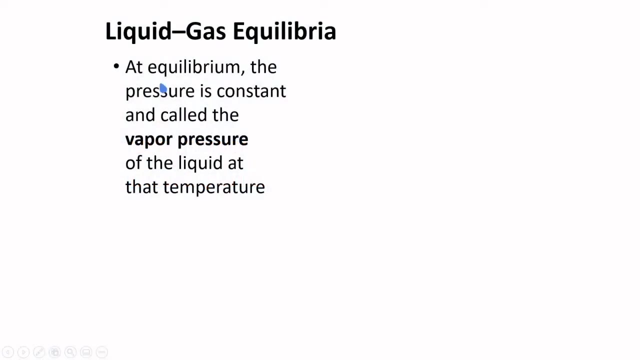 At equilibrium, the pressure is constant and is called the vapor pressure of the liquid at that temperature. If we place a liquid in a vacuum, evaporation will start, and at this point the rate of vaporization is greater than the rate of condensation. As time progresses, there will 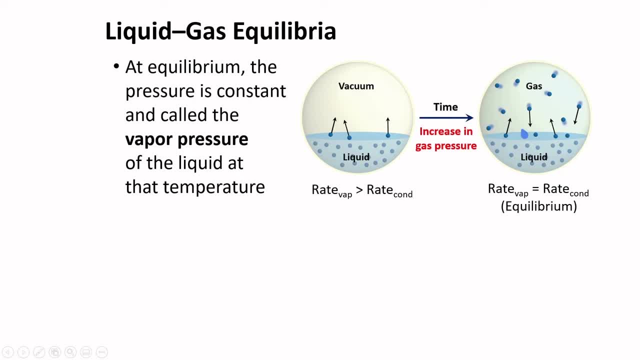 be more particles in the gaseous state and ultimately there will come a point where the rate of vaporization is equal to the rate of condensation. This point is at equilibrium and the pressure exerted by the gas is called the vapor pressure. Vapor pressure is proportional. 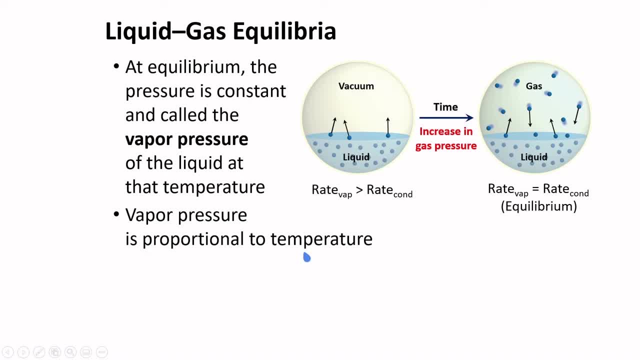 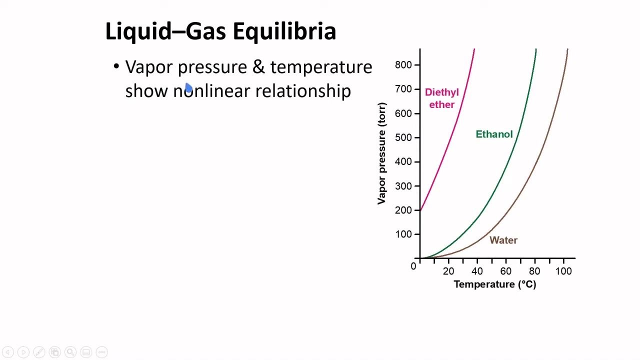 to temperature. The higher the temperature, the greater the gas pressure or the vapor pressure. The weaker the intermolecular forces of the substance, the higher the vapor pressure. The plot of vapor pressure and temperature show nonlinear relationship. The Clausius-Clapeyron equation converts this nonlinear. 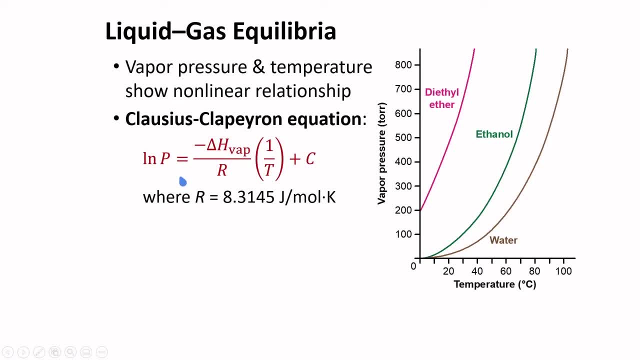 relationship into a linear one, where R is the universal gas constant, 8.3145 Joules per mole per Kelvin. Again, this is a linear equation and if two points are taken, we can have this new formula and this will allow us calculations of pressures and temperatures. 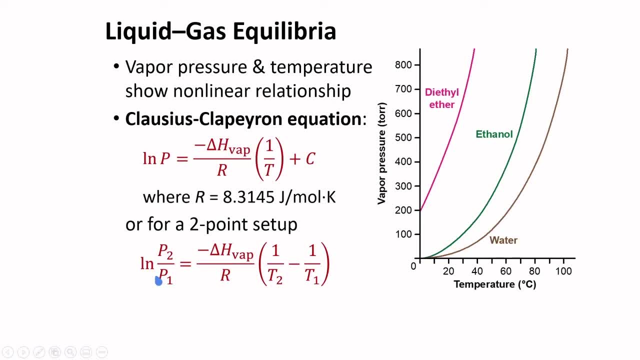 If the other points are given, Boiling point is the temperature at which the vapor pressure equals the external pressure. If the external pressure is 760 Torr, this is equal to one atmosphere. then we can have the normal boiling points of substances. For diethyl ether, this is at 34.2. 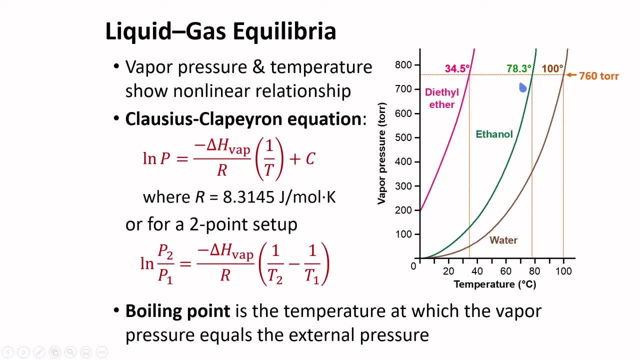 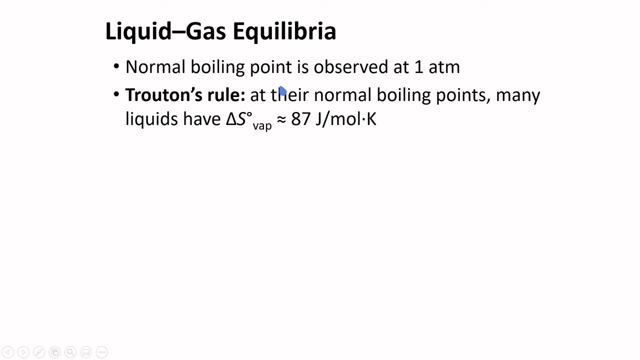 4.5°C, for ethanol 78.3°C and for water 100°C. You will also notice here that at any given temperature the less polar diethyl ether has the highest vapor pressure of the three substances. Normal boiling point is observed at 1 atmosphere. 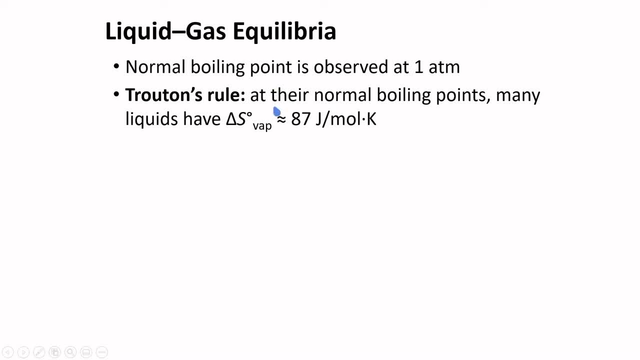 We also have Troughton's rule, which states that at their normal boiling points, many liquids have an entropy of vaporization approximately equal to 87 Joules per mole per Kelvin. This may be used to estimate the heat of vaporization of liquids with known boiling points. 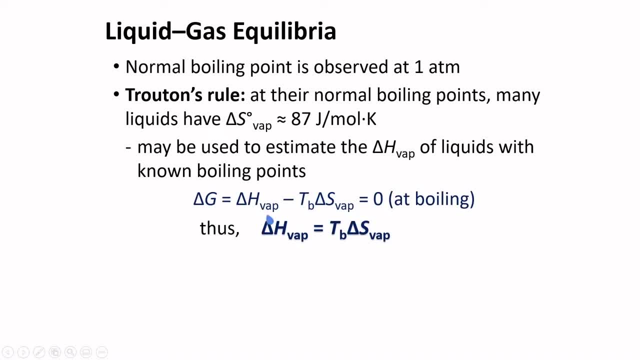 As you know, the temperature of vaporization of liquids with known boiling points is approximately equal to 87 Joules per mole per Kelvin. Boiling of substances is an equilibrium condition, and so delta G, the change in Gibbs free energy, is equal to zero. 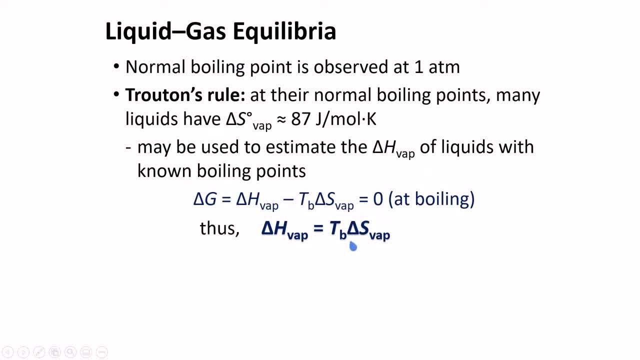 Hence we can rearrange this formula into this one. If delta S of vaporization is equal to 87 Joules per mole per Kelvin and the boiling temperature is known, We can have an estimate of the heat of vaporization. Take note that those liquids with significant special interactions, for example hydrogen, 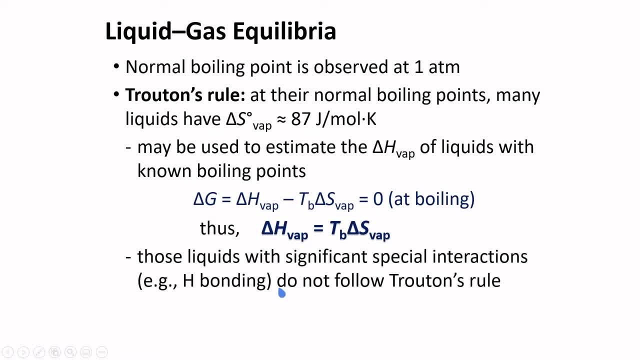 bonding do not follow Troughton's rule. Water, ethanol, formic acid and hydrogen fluoride do not follow this rule. This is the result of the following analysis. This is the result of the analysis. This is the result of the analysis. 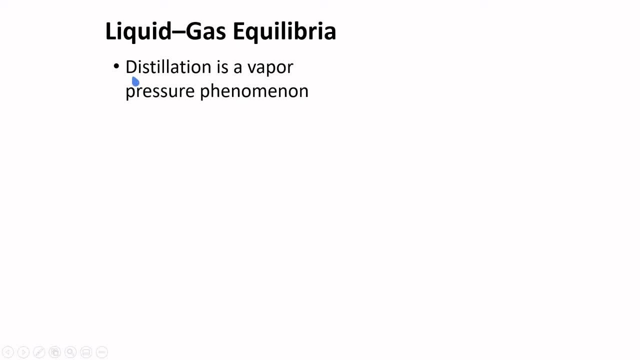 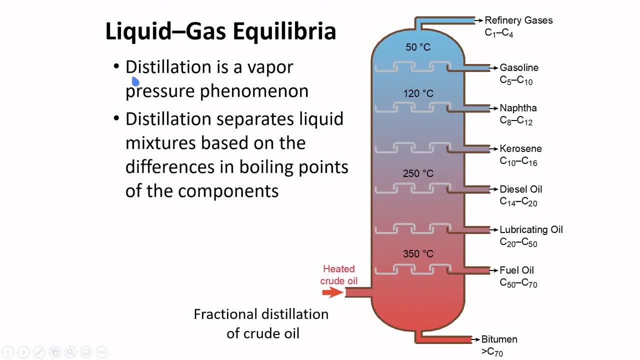 This is the result of the analysis. Distillation is a vapor pressure phenomenon. Distillation separates liquid mixtures based on the differences in boiling points of the component. A good example here is the fractional distillation of crude oil. As heated crude oil passes through this system, the vaporized crude oil can condense at different 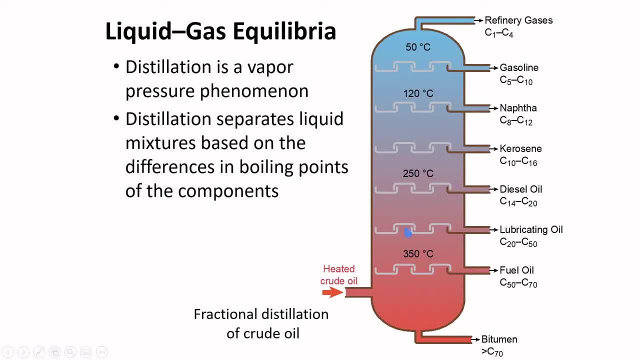 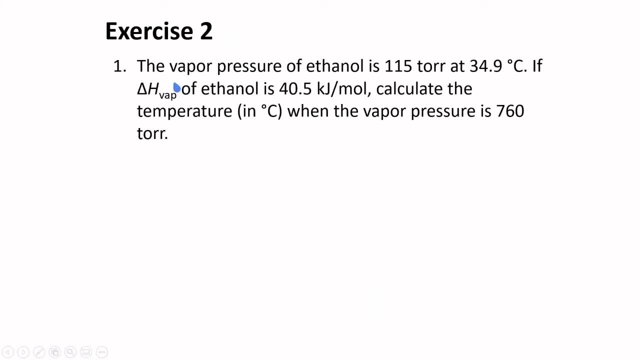 temperatures they can be separated. exercise 2: the vapor pressure of ethanol is 115 Torr at 34.9 degrees Celsius. if the heat of vaporization of ethanol is 40.5 kilojoules per mole, calculate the temperature when the vapor pressure is. 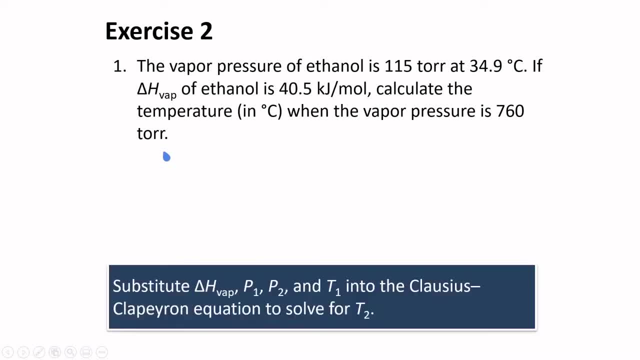 760 Torr. here we can use the Clausius Lapeyron equation. P1 and T1 are given, that is, 115 Torr, and 34.9 degrees Celsius. P2 is also given, that is 760 Torr. what is required is T2 if we rearrange this equation. 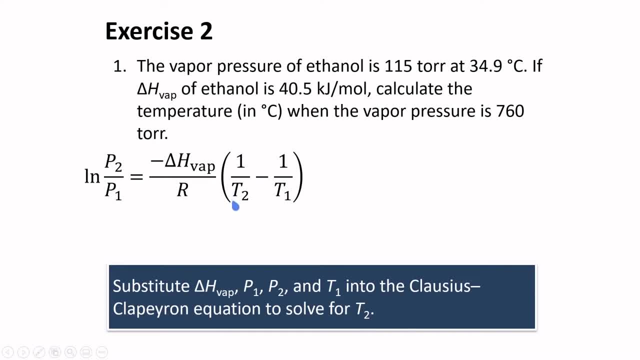 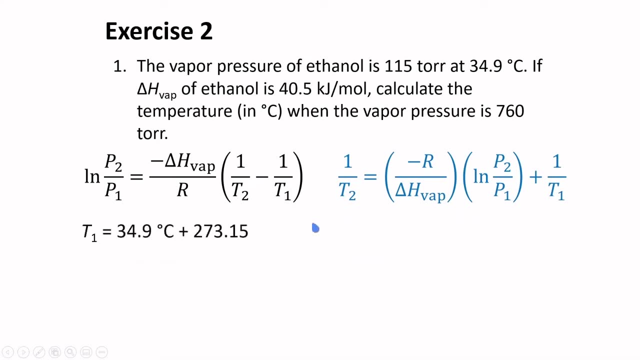 such that this term here is placed on the left side, we will get this new relationship. T1 is in degrees Celsius, so we need to convert it to Kelvin. just add 273.15 to that value and you will get 308.0 Kelvin. just need to plug in all. 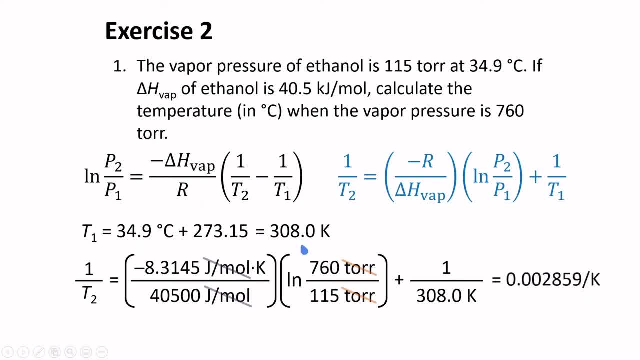 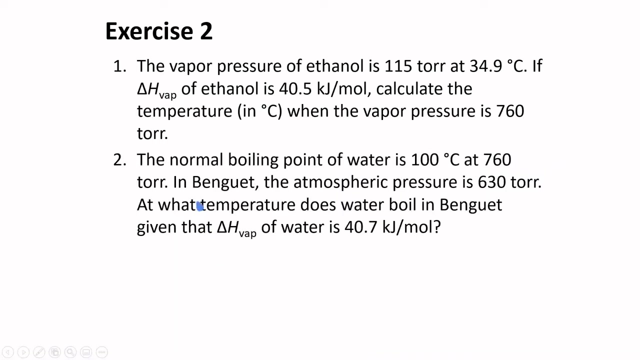 the values. cancel all the units and we will get 0.002859 per Kelvin. taking the inverse of this relation, 349.8 Kelvin is obtained. this is equivalent to 76.6 degrees Celsius. the normal boiling point of water is 100 degrees Celsius at 760 Torr in. 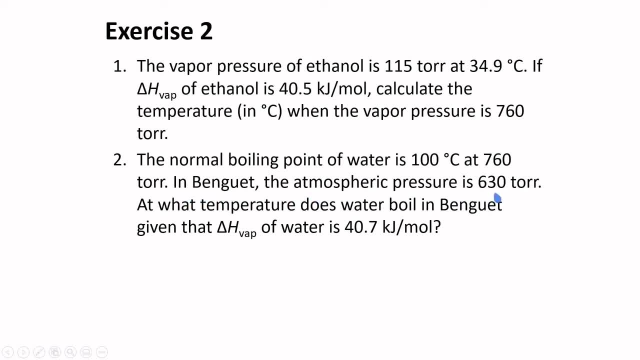 Benguet the atmospheric pressure is 630 Torr. at what temperature does water boil in Benguet? given that the heat of vaporization of water is 40.7 kilojoules per mole, I will leave this question for you to answer. the procedure is very similar to item number one. 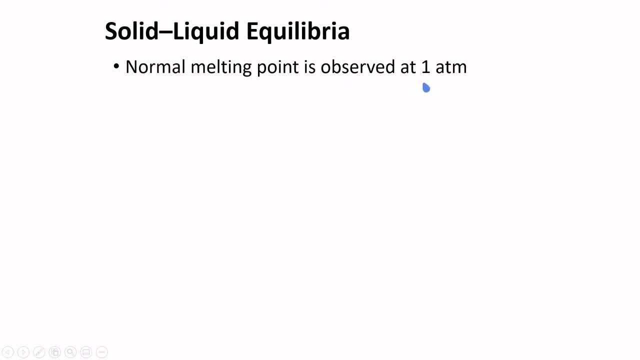 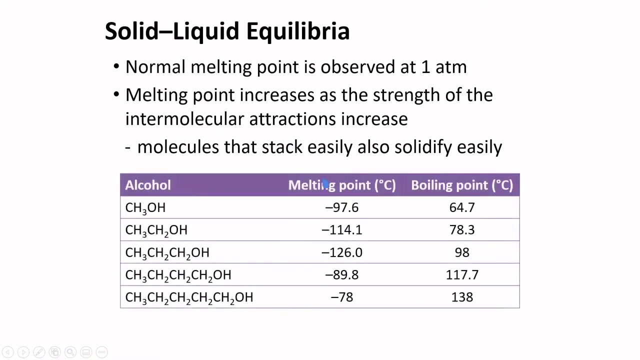 normal melting point is observed at one atmosphere. melting point increases as the strength of intermolecular attractions increase. molecules that stack easily also solidify easily. consider the melting and boiling points of these alcohols. with increasing number of carbons here you will see that boiling point increase as the number of carbons increase. 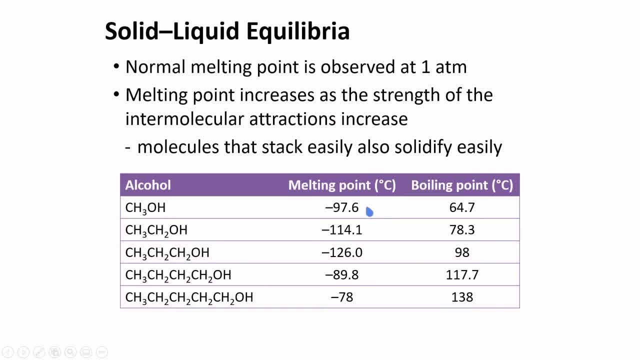 if you compare the melting points, there is a decrease in value as we go from methanol to ethanol, to propanol. for the four carbon butanol, the melting point increases and the increasing trend is maintained by the five carbon fentanyl. what is going on here? 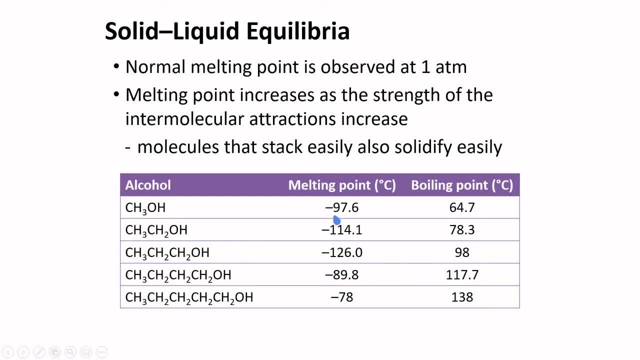 the stacking could be the reason. generally, we would expect the melting point to increase the same way as boiling point does. this unusual downtrend can be attributed to the stacking or packing of the solids. propanol is probably packed less efficiently compared to methanol, so it can easily melt. 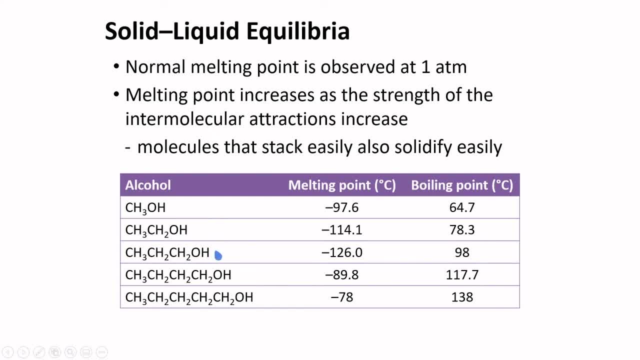 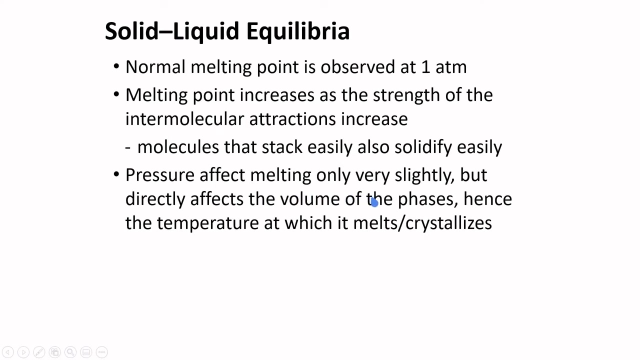 the non-polar carbon chain disrupts the hydrogen bonding Network as the solid is formed. as more carbons are added, intermolecular attractions increase, which are related to the increase in molar mass, and they become dominant, increasing the trend in melting point. pressure affect melting point only very slightly. 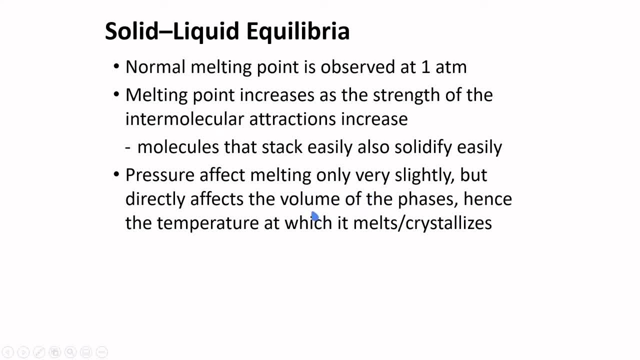 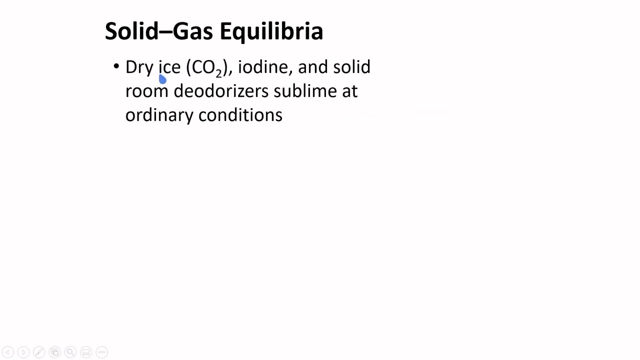 but directly affects the volume of the phases, hence the temperature at which it melts or crystallizes. we can use here the Clapeyron equation. in this equation, Delta V of fusion is equal to the volume of the liquid minus the volume of the solid and the volume of the liquid minus the volume of the solid. 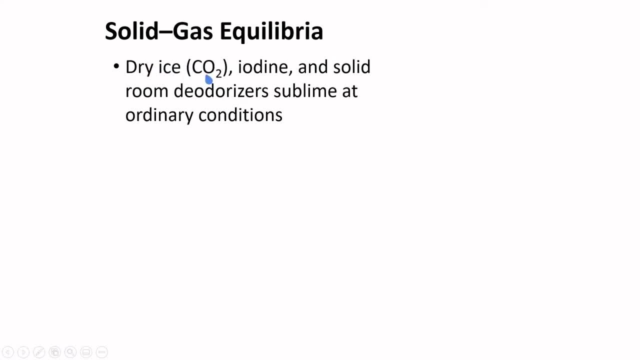 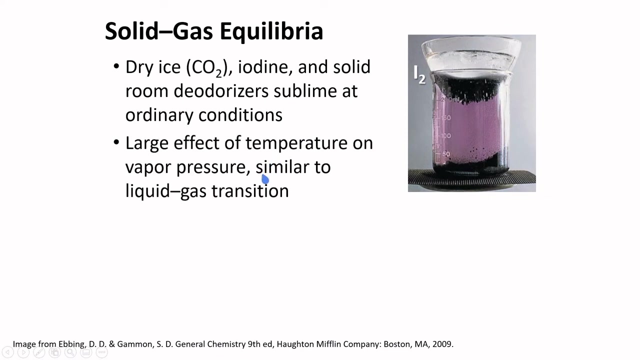 Dry ice or solid carbon dioxide, iodine and solid room deodorizers sublime at ordinary conditions. you can see the sublimation here. in the case of iodine, there's a large effect of temperature on vapor pressure and this is similar to liquid to gas transition. 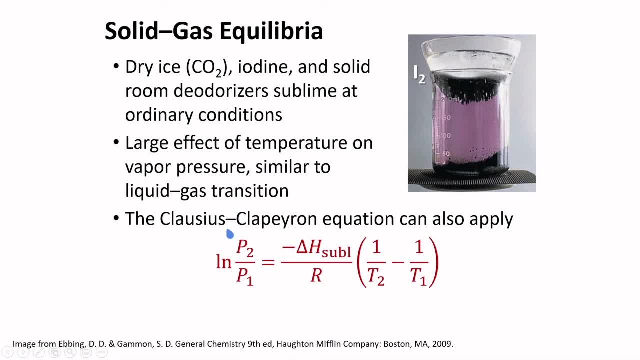 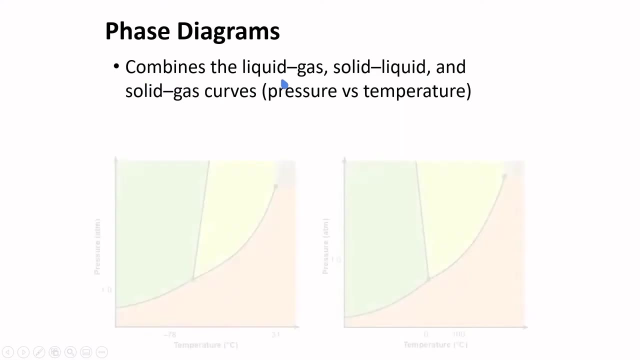 For solid gas equilibria, the Clausius-Clapeyron equation can also apply, but instead of the heat of vaporization, the heat of sublimation is utilized. Phase diagrams combine liquid-gas, solid-liquid and solid-gas curves, and this is a graph. 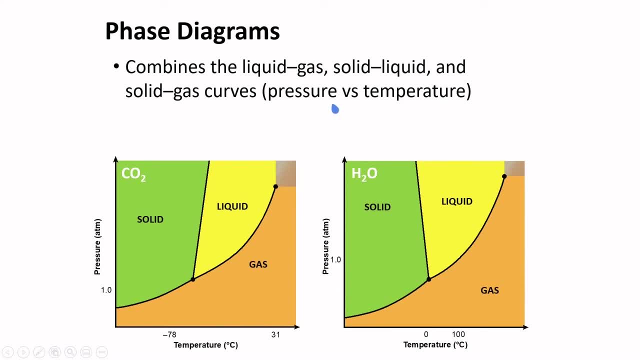 of pressure versus temperature. It shows regions of each stable phase and the lines corresponding to phase transitions. In phase diagrams we can determine specific points of corresponding temperatures and pressures At one atmospheric pressure and negative 78 degrees Celsius. solid carbon dioxide transitions to a gas. 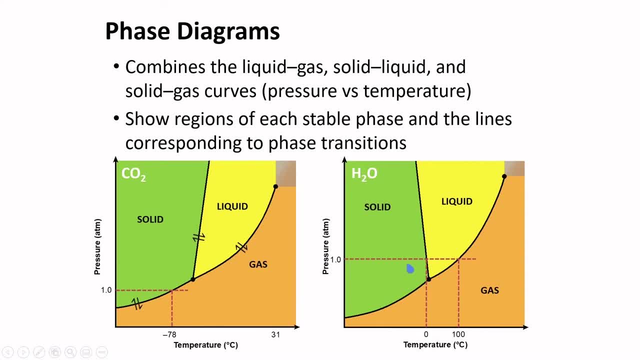 Solid water, on the other hand, will be converted at zero degrees Celsius to a liquid and then to a gas at 100 degrees Celsius. Note that water expands on freezing, causing the solid to be less dense than the liquid. The increase in pressure favors the phase that occupy less space. 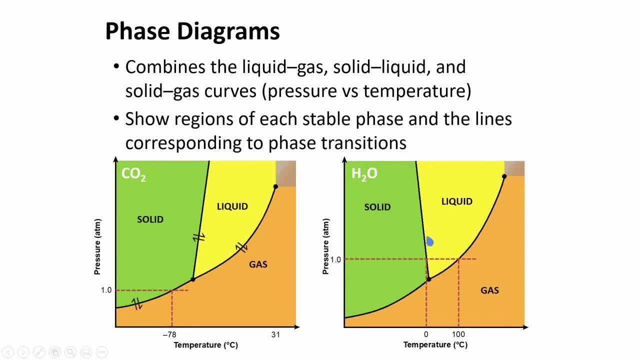 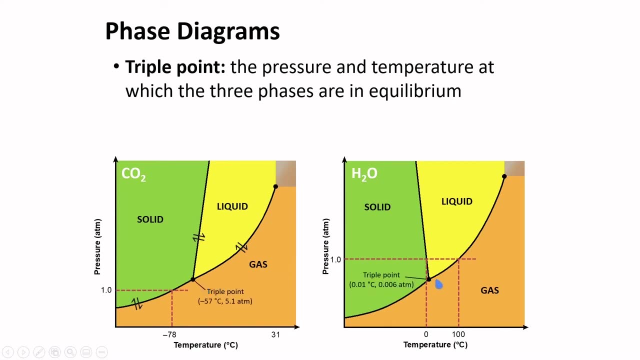 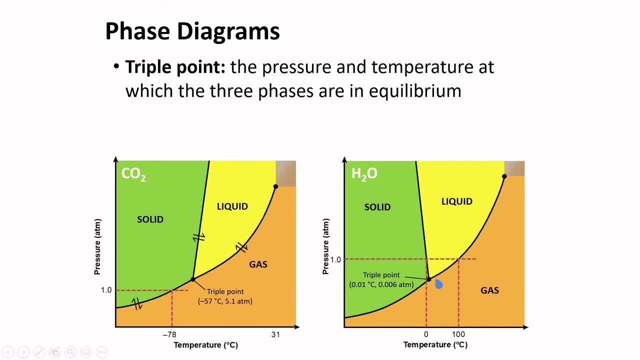 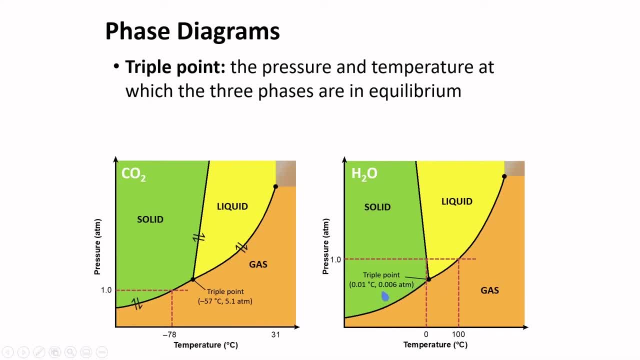 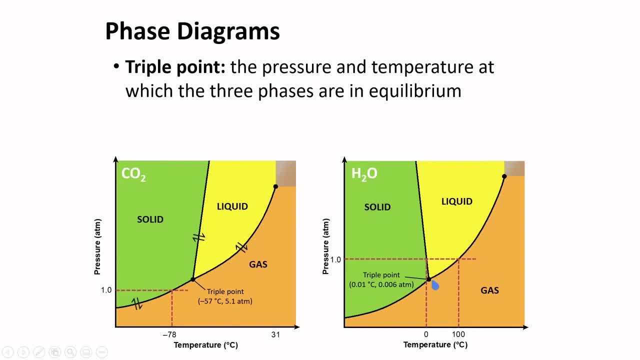 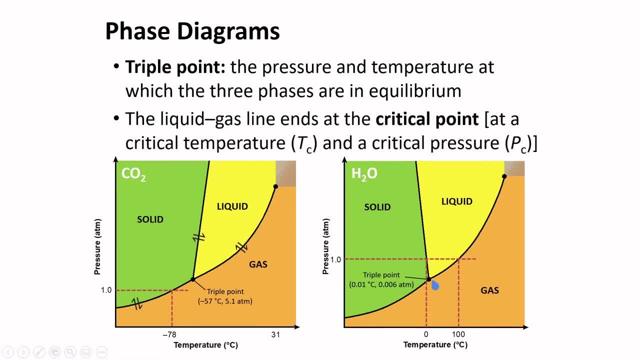 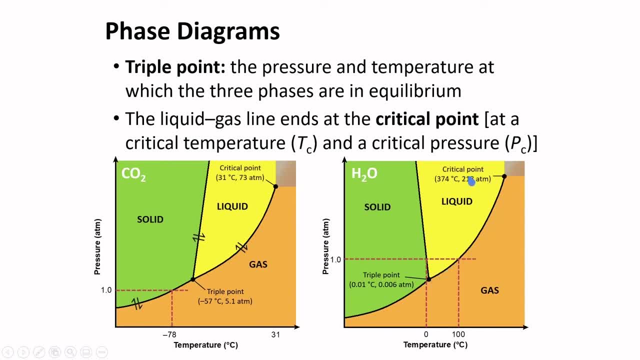 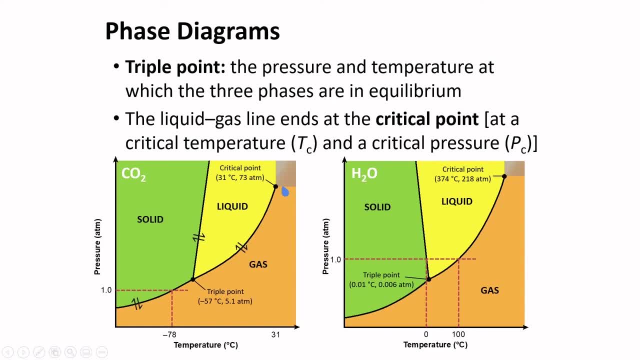 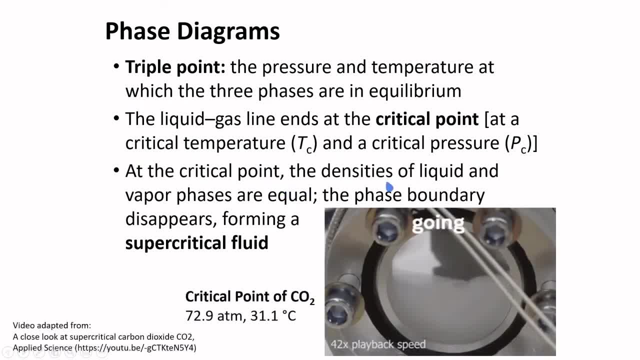 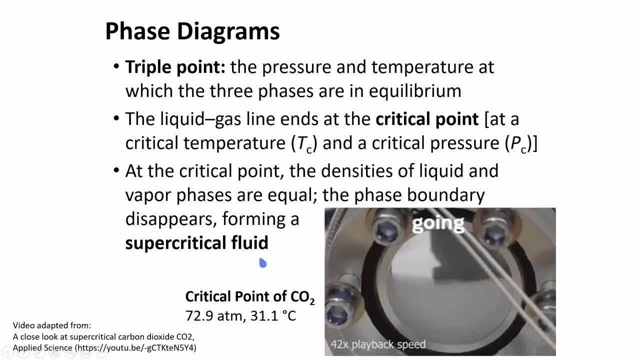 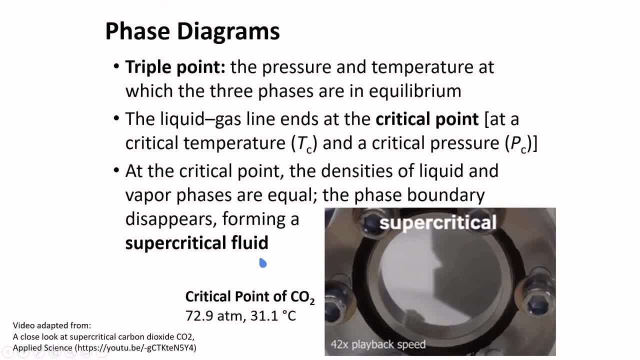 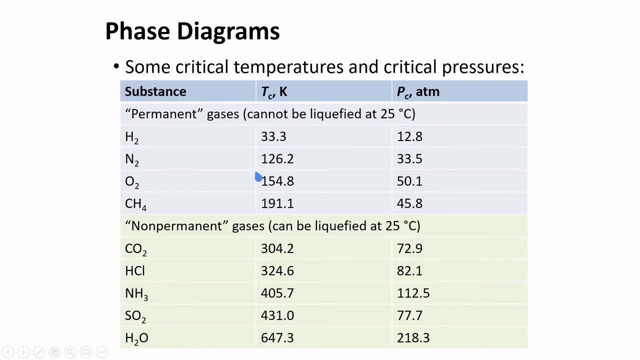 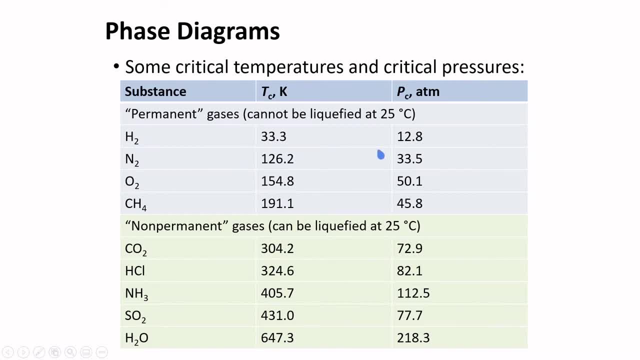 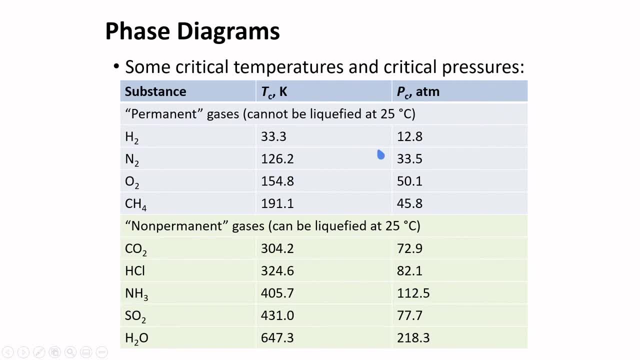 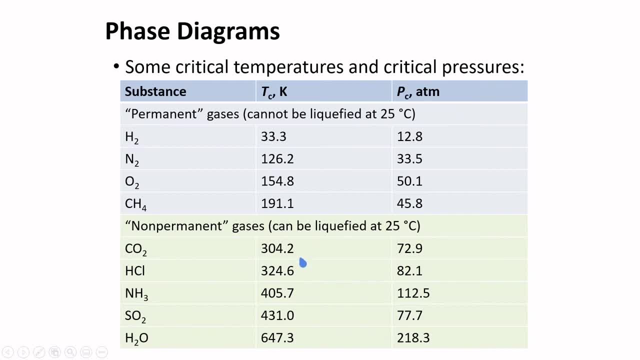 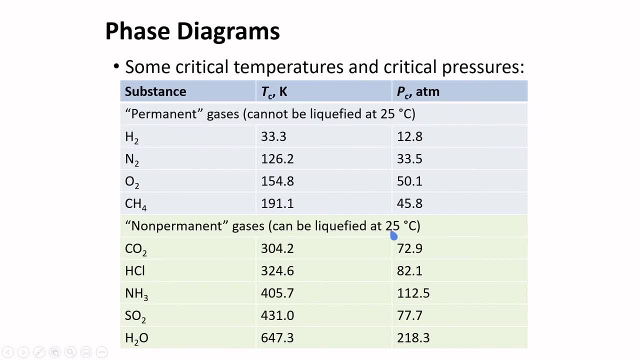 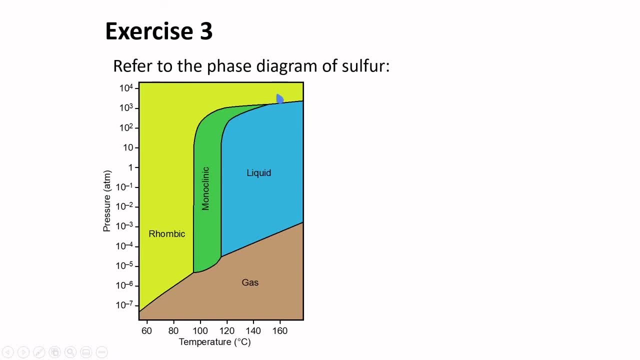 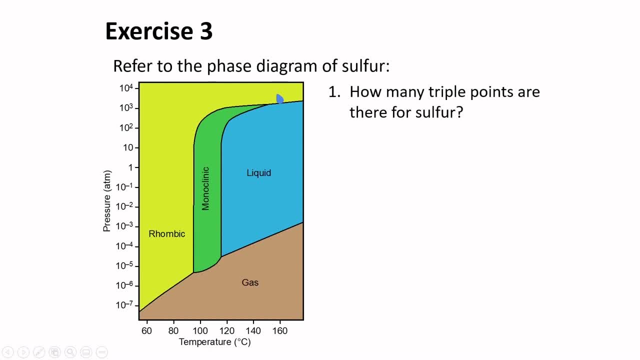 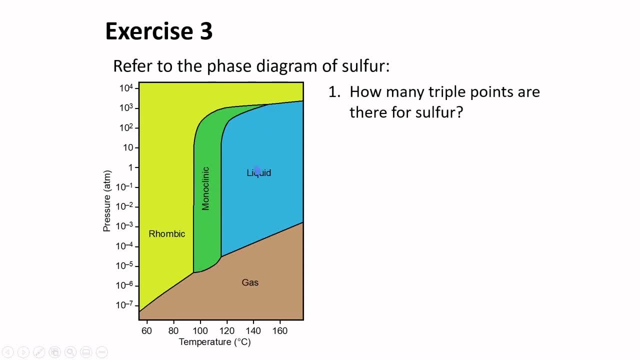 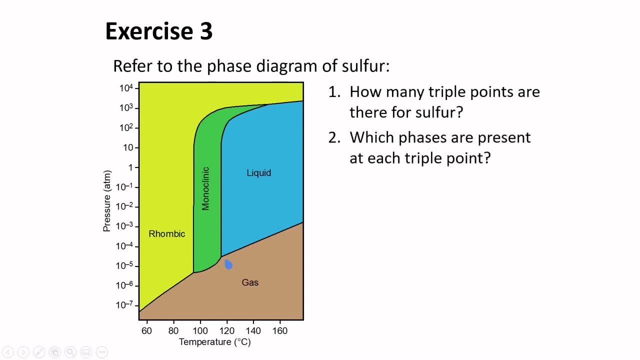 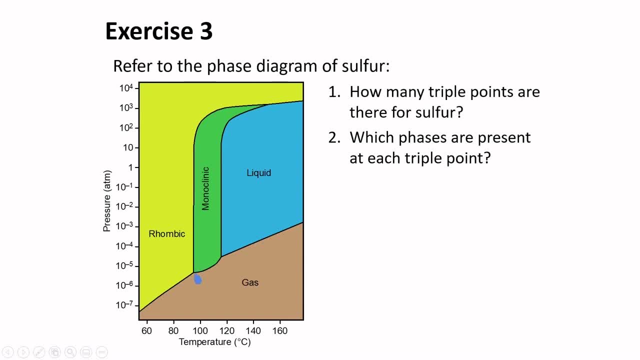 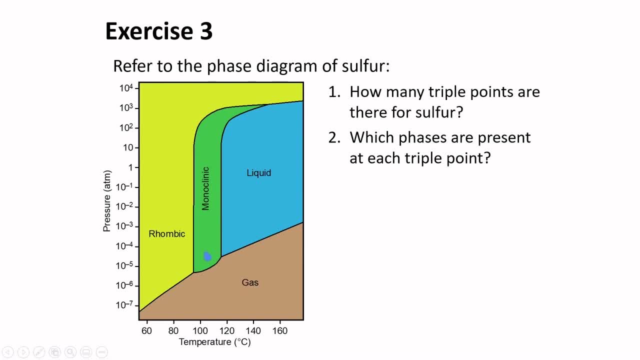 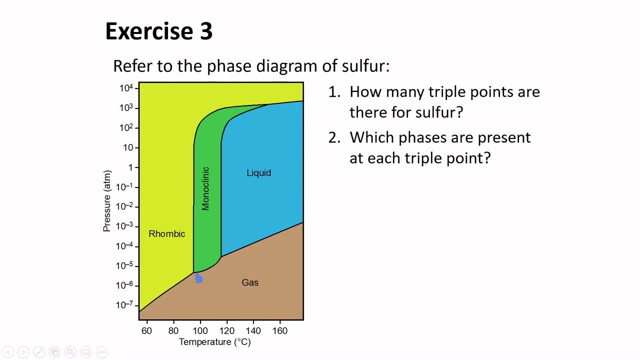 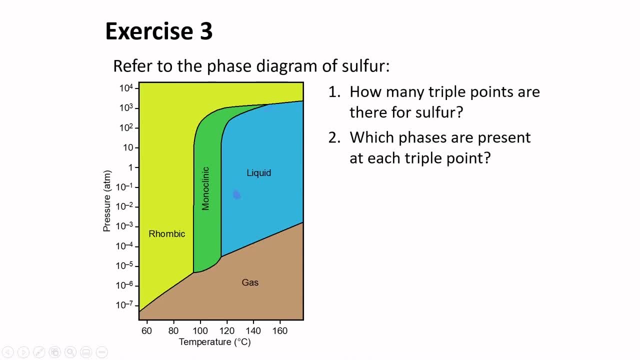 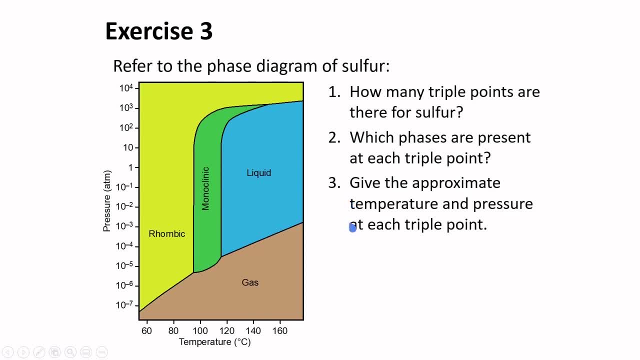